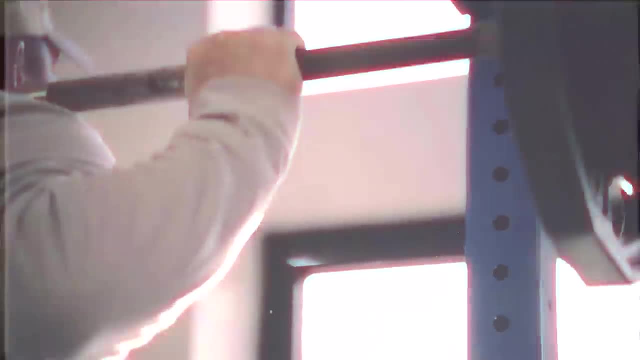 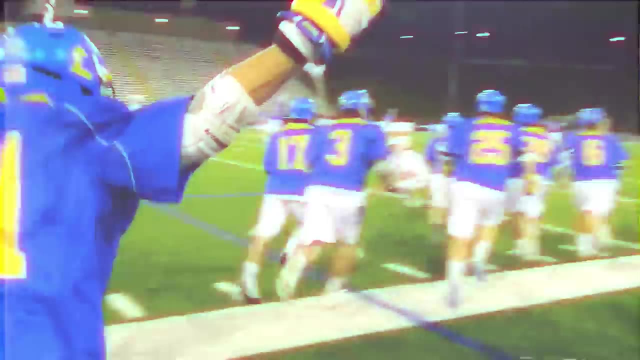 St Joseph's team upset St Mary's to let Loyola slide into the sixth and final seed of the conference playoff. The Dons do have some momentum on their side, though. They just crushed second-seeded McDonough by a score of 13-4 just a few days ago. 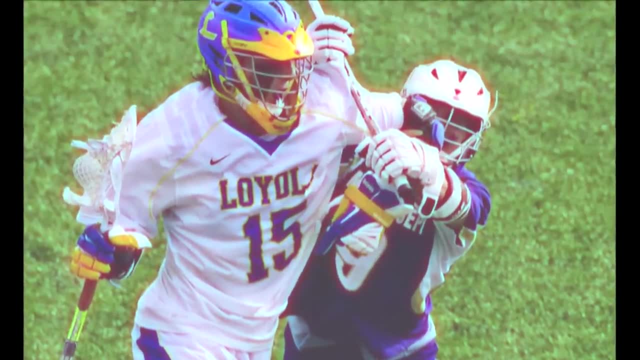 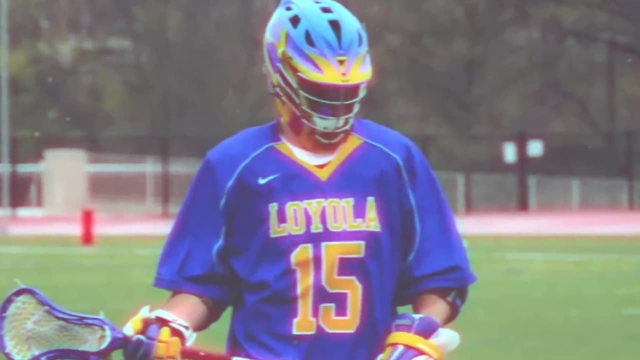 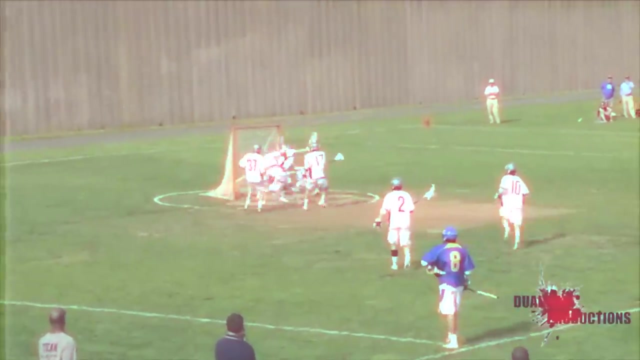 They also have Ryan Conrad, the number one ranked sophomore in the country. He's an athletic do-it-all midfielder headed to Virginia in 2015,, and he needs to have a big game. Loyola also has Devin McNamara, a senior Villanova commit, who uses his high lacrosse IQ to pick apart defenses. 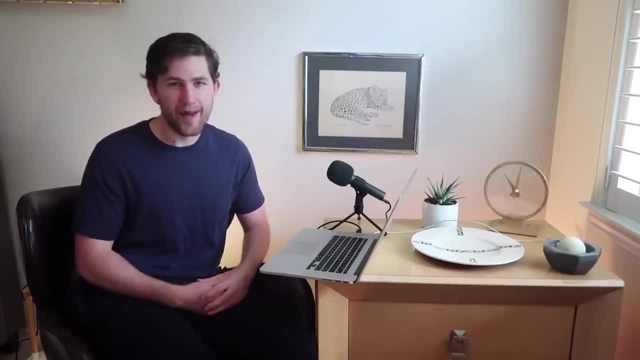 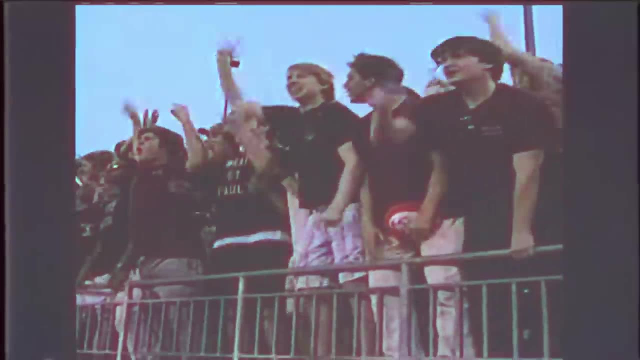 So here we go. Boys Latin, the undefeated team that many are calling the greatest ever, versus Loyola, the underdog, who's pretty lucky to be here right now. The crowd at Johnny Unitas Stadium is electric and ready to go. Two teams are looking for. 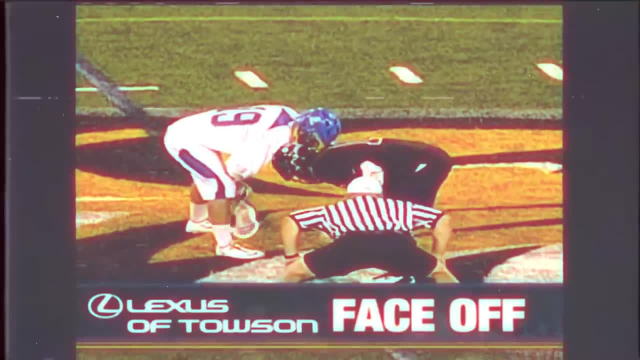 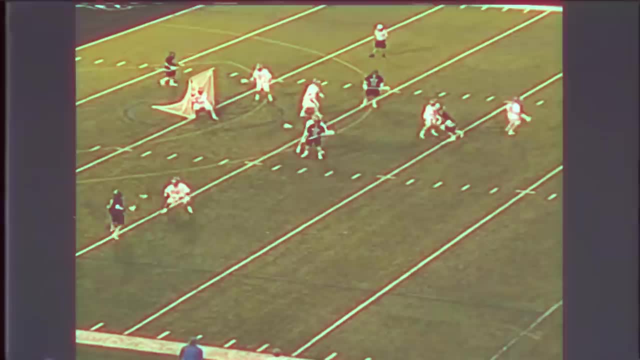 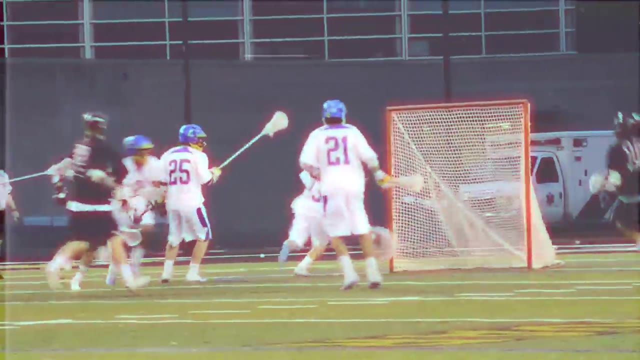 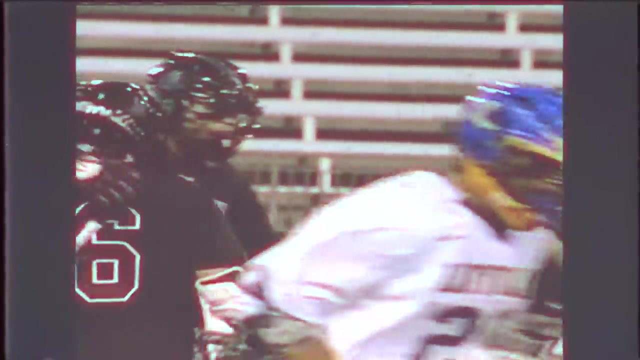 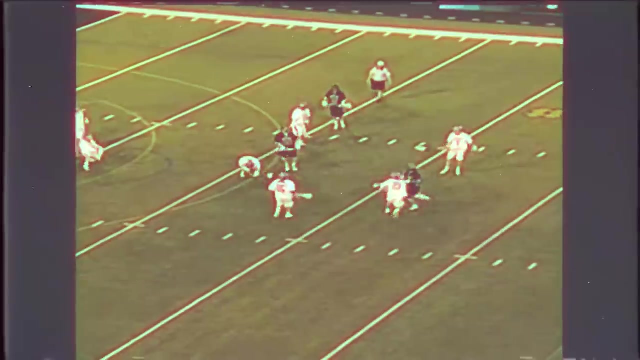 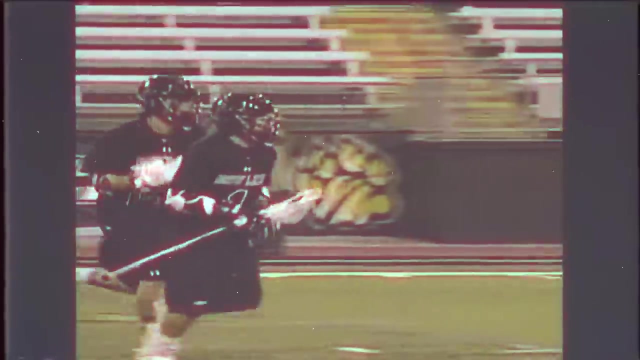 glory and one game will decide it all. BL would love to make it a 2-0 game. There's a shot and that's exactly what happens: Scoring for Boys, Latin Keegan O'Connor- and they suddenly have a 2-0 lead. 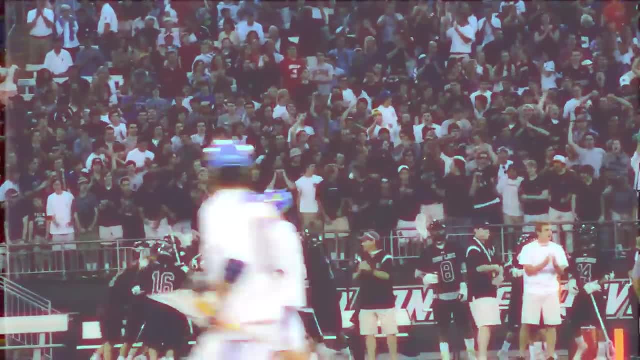 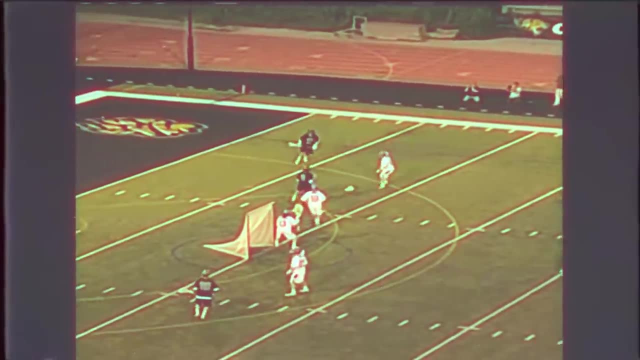 So BL with the 2-0 lead here in the MIAAA Conference Championship. I don't see a lot of stress down there, Bugs. They look very, very calm, They're very calm. and you know one thing that you don't see a lot at the high school level: that 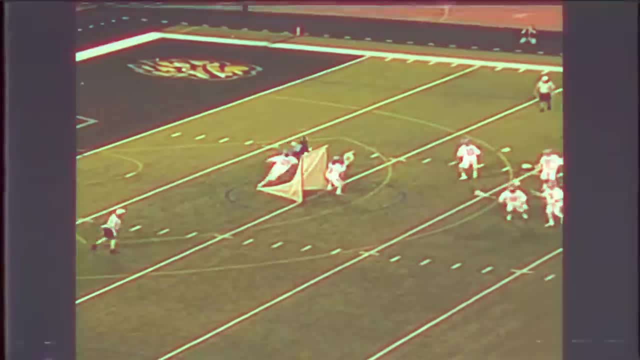 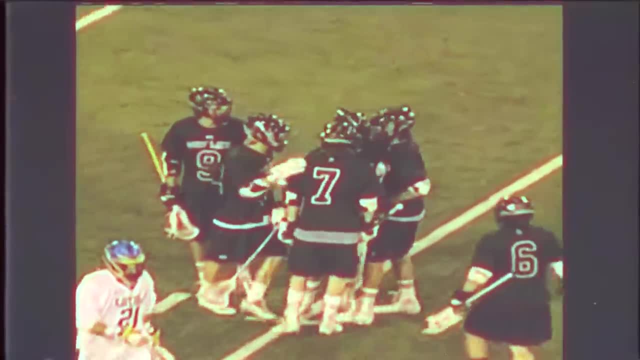 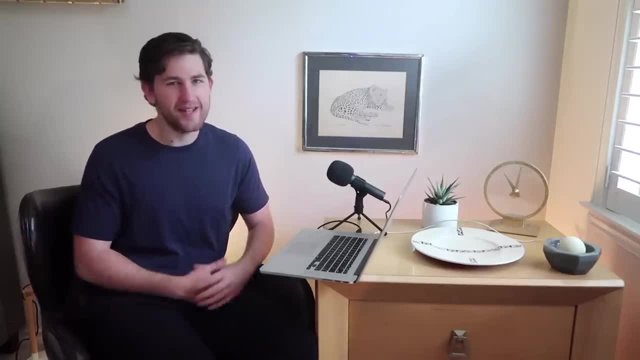 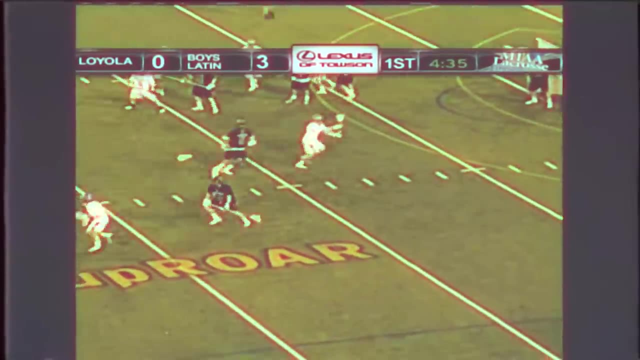 Okay, it's 3-0. Boys Latin and we're not even close to being done with the first quarter. This game could get ugly fast. Tim Nordbrook now Nordbrook looking for some space, Couldn't find it. BL's playing at defense. 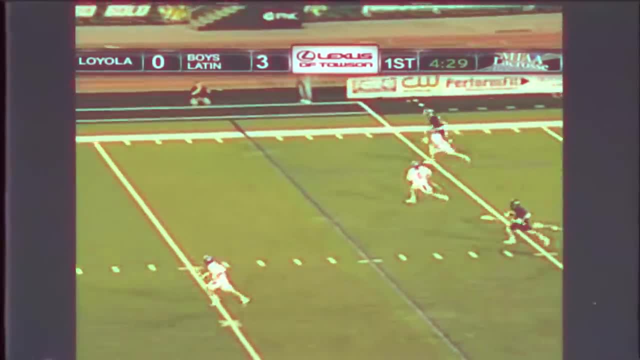 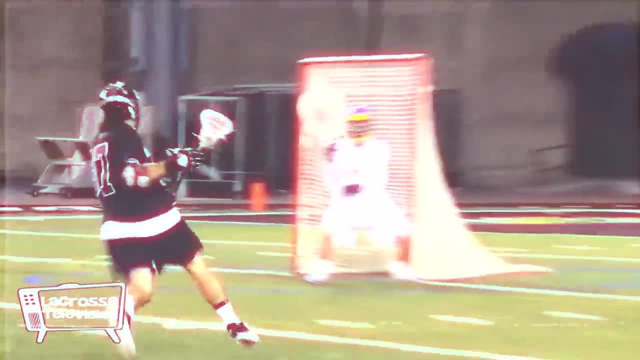 Man Ball's loose and BL's right there, That's Talley. Bruno Picked up the loose ball, Bruno taking it in himself, and he scores. How about that? That's a great Front end and the back end Bucs. 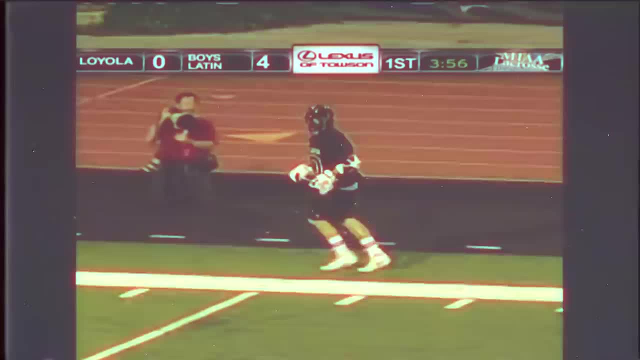 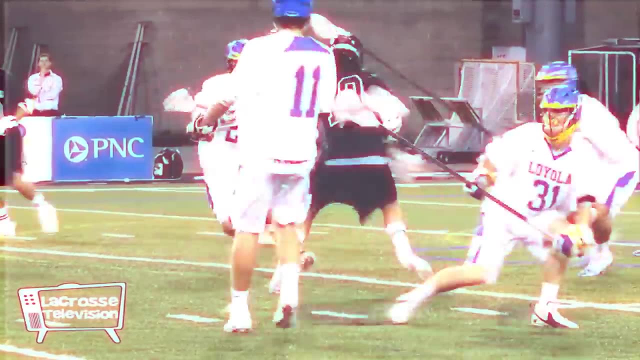 Coast-to-coast play Does a great job, Picks the ground ball up. As Bucs just pointed out, they were defeated in the semi-finals the last two years in a row. so this MIAA championship, especially by their senior class, sorely wanted. And look at that. 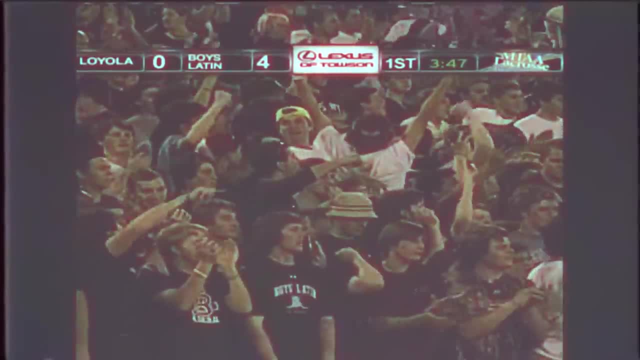 Just weaving his way through the defense. That's Colin Heacock. That's. that's a great individual effort by Colin Heacock. The Dodgers are going to win this game. That's a great individual effort by Colin Heacock. The Dodgers are going to win this game. 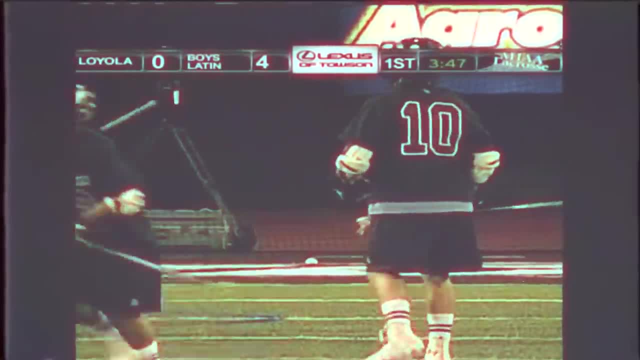 That's a great individual effort by Colin Heacock. The Dodgers are going to win this game. That's a great individual effort by Colin Heacock The Dodgers. man Tucks his stick, So here come the Lakers: 2.50 to go in the first quarter. 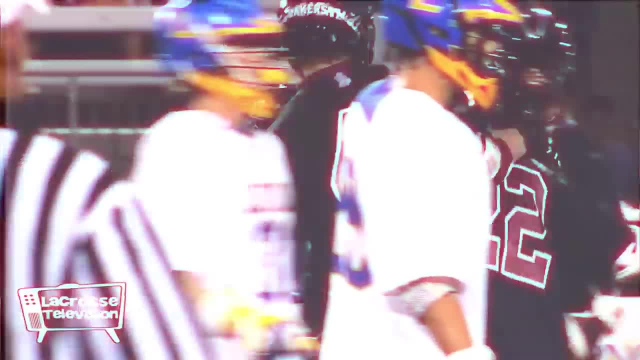 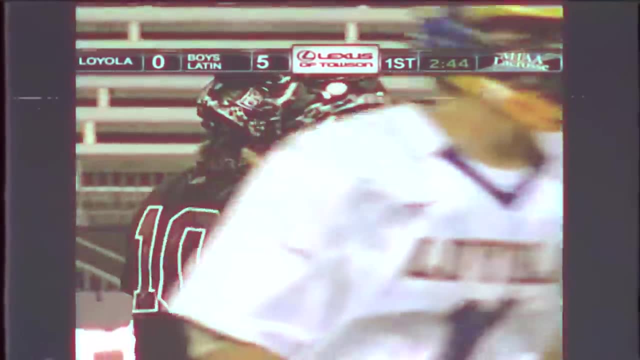 And again, Give that one to Colin Heacock Bucs. they're not running plays, They're not setting picks, There's no assist. I've never seen anything like this. Boys Latin is showing us why they're the number one team in the nation. 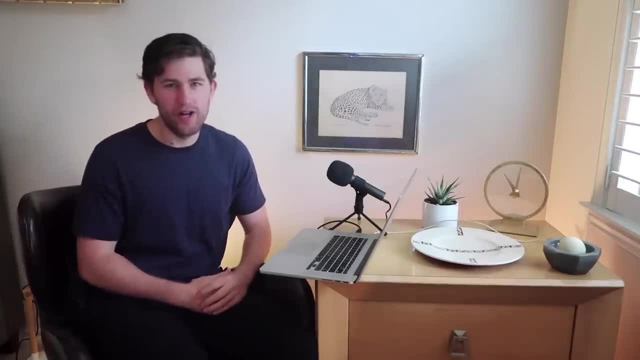 They're making plays all over the field and killing loyals. They're making plays all over the field and killing loyals. They're making plays all over the field and killing loyals. Colin Heacock already has a hat trick And his strength and power is unguardable. 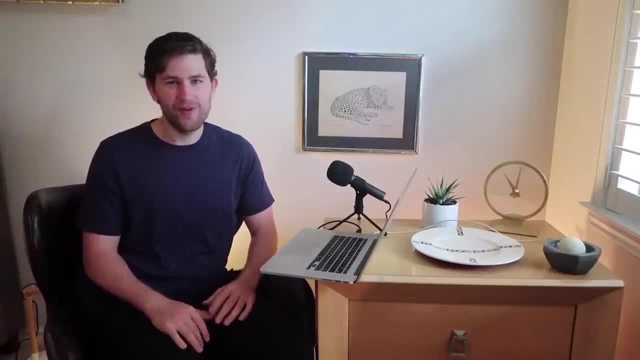 And his strength and power is unguardable. Loyola isn't getting any good looks on offense, and this quarter couldn't be going any worse. Loyola isn't getting any good looks on offense, and this quarter couldn't be going any worse. 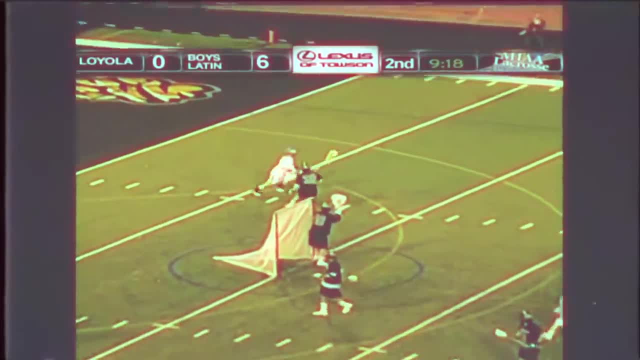 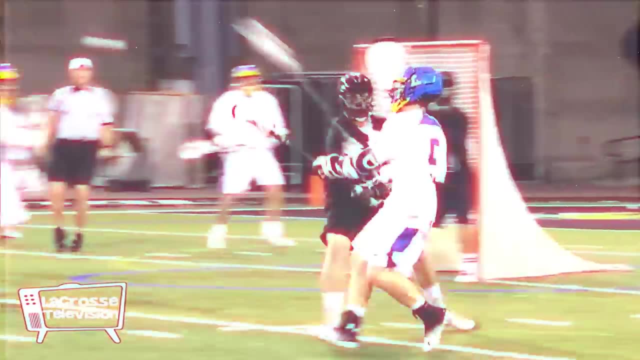 It's on the high school recruiting game, which is just growing in leaps and bounds. We covered players from all across the country. We're going to be big stars at division one. So for Loyola crossing, that was Tim Northbrook, but we've got a flag. 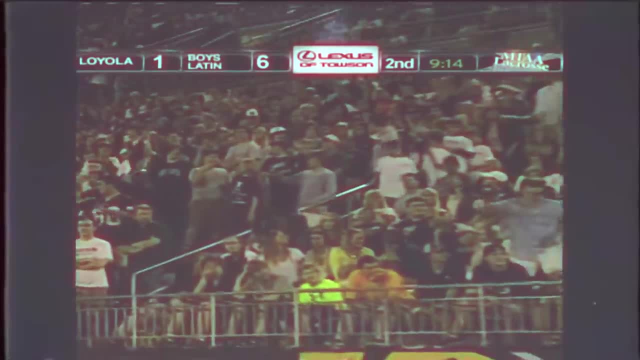 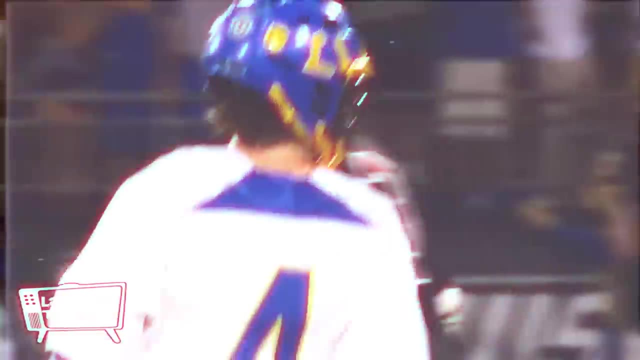 Loyola apparently has gotten onto the scoreboard. Yes, they have. Loyola has gotten onto the scoreboard. Yes, they have Read that publication you need to Inside. Lacrosse does an outstanding job and has for a good many years. They scored again. Dead Loyola, That will be Devin McNamara. 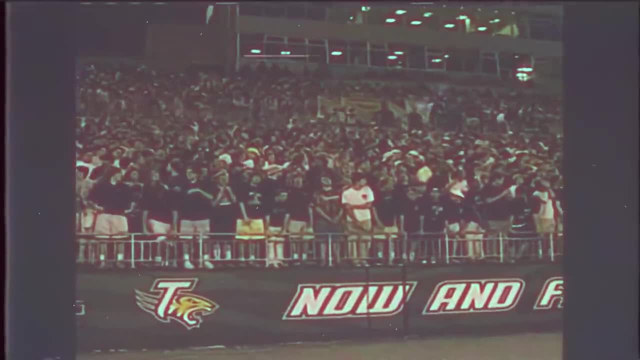 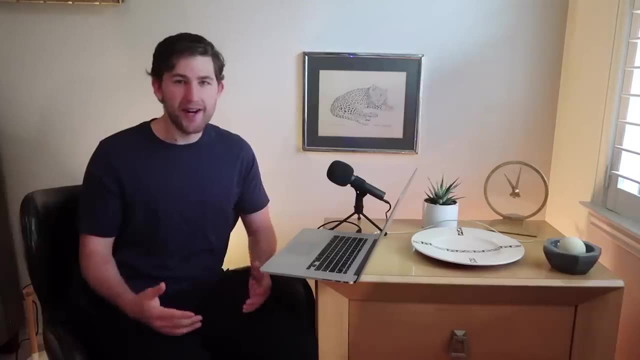 Bucks. we talked about runs and it looks like Loyola's on a run. They need a run here. They get two goals in a row. They get a goal here by Devin McNamara, who's really been the catalyst, But the Dons show their resiliency. They get two quick goals. 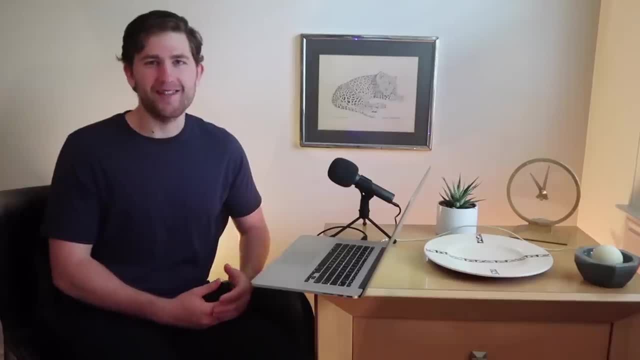 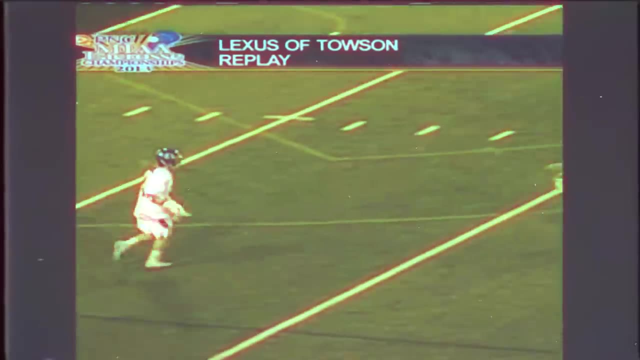 Now Loyola is settled in, Their defense is making stops, Their offense is finding gaps. This is a completely different game than just a few minutes ago. He simply beats his man, which he hasn't done yet today, and they haven't had to slide, so they don't really slide. 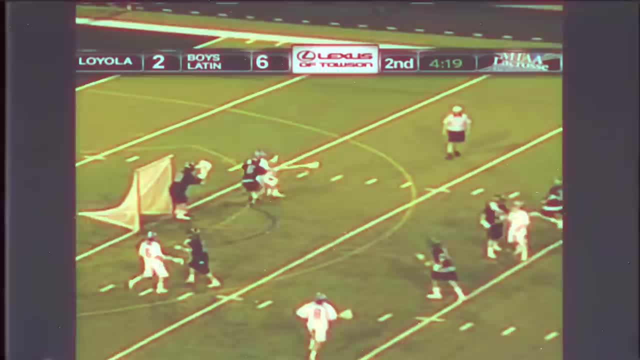 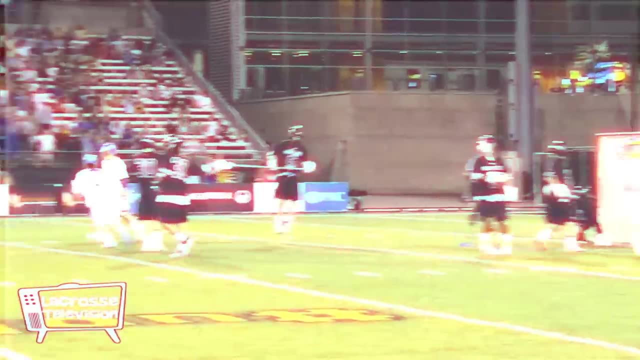 And he puts a nice, keeps a stick next to his ear, puts it high to low in a good spot. Bob's going to Maryland, Ryan Conrad going to Virginia. so this will probably be a matchup for years to come. Virginia loves those Baltimore kids, don't they? And there you go, that's Conrad. 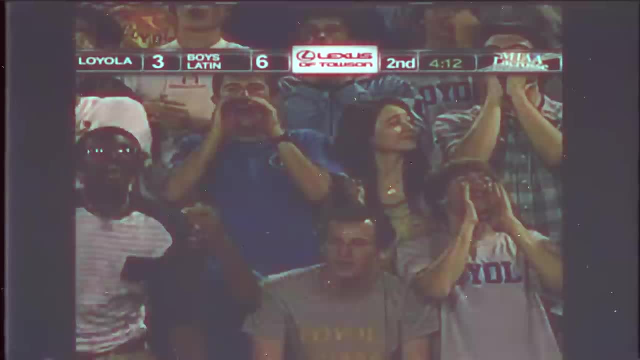 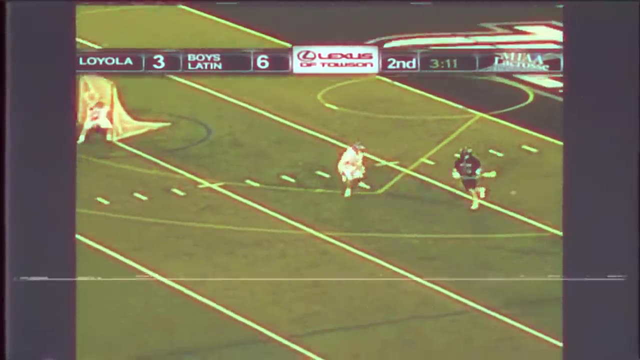 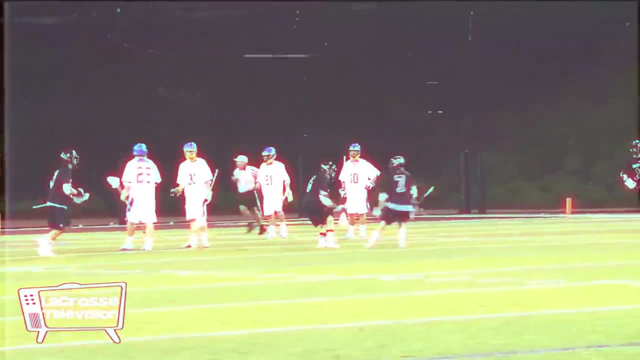 Battling the defense. Bender turned, planted. his foot went low. So yeah, you're hearing some life from the Loyola side of the field right now. You're going to want to put the ball in their stick- Definitely are. So here we go. Here's BL again, And again AC Newton gets beat. 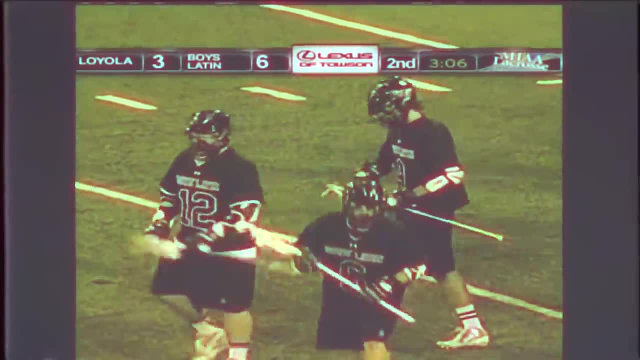 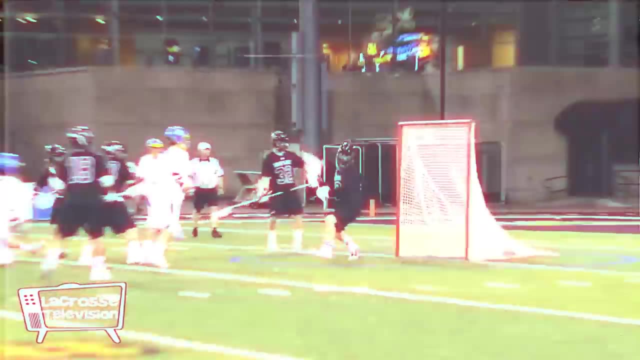 So that's a great shot there. That was Michael Lynch for Boys Latin. It's nice to see some newer names come up in the B and C Conference, isn't it? Definitely some new schools getting the MIA and becoming successful. 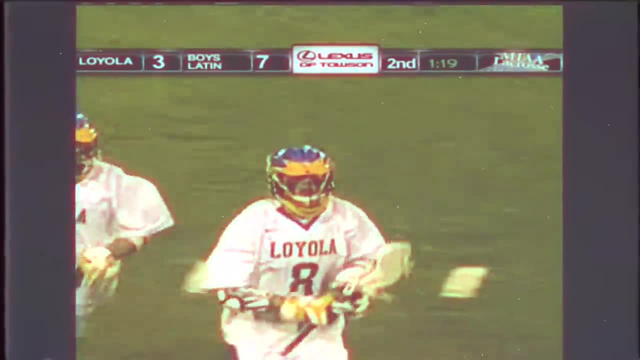 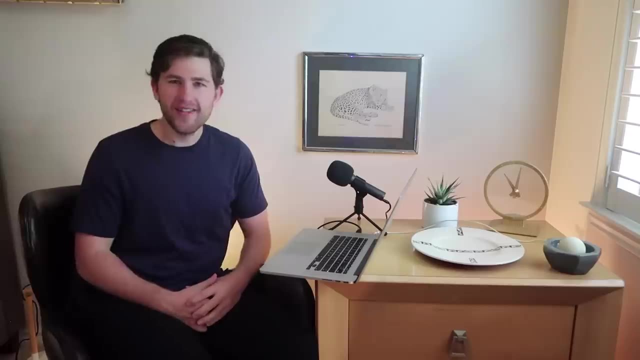 Cutting across the front for Loyola. That was Tyler Luella and he got a nice assist from Devin McNamara And, as you said, McNamara is one of the guys that's got to make a goal. The teams are trading goals back and forth and it's 7-4 at halftime. 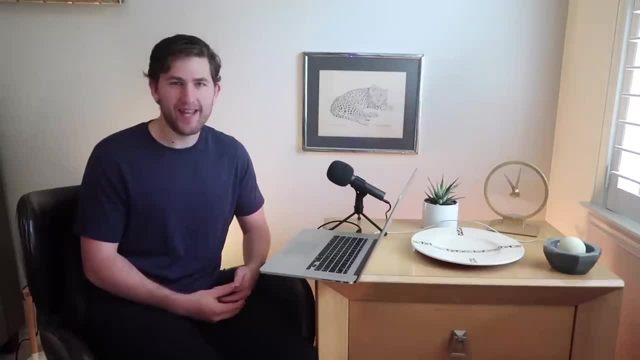 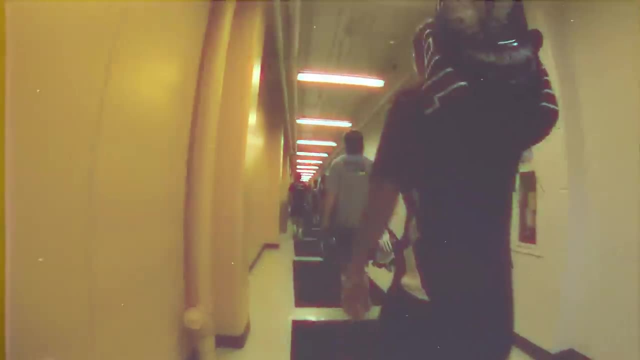 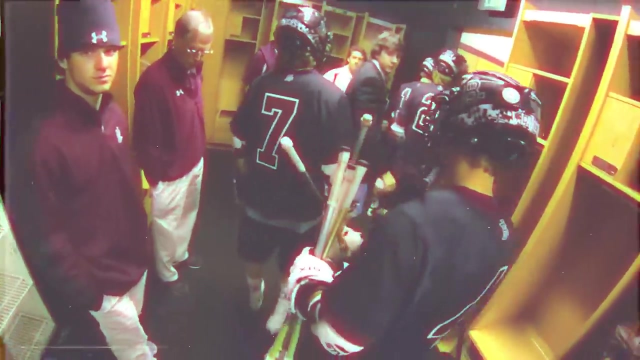 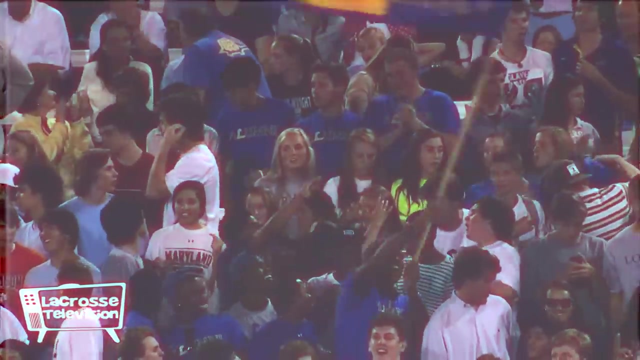 Loyola has been responding well, but a three-goal deficit against Boys Latin won't be easy to crack Both squads, head into the locker room and strategize for the next game. We'll see you guys in the next half. Here you go. They see them dodging on a short stick. 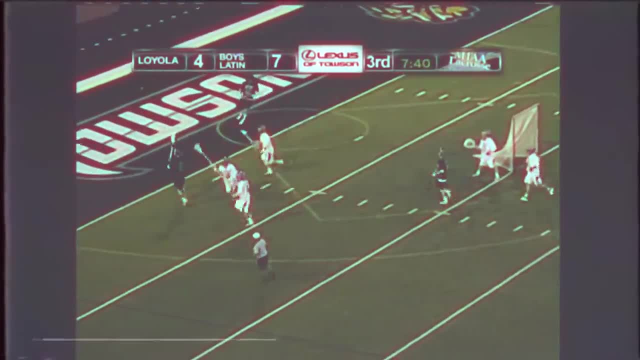 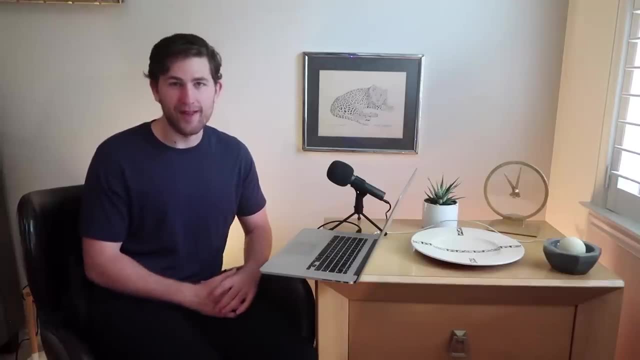 Here comes Stanwyck, Ran into some tough defense And look at Loyola, just swarm. And I guess that's Right now. both teams are playing lockdown defense, Loyola goalie AC Newton is heating up And neither team's offense has answers right now. 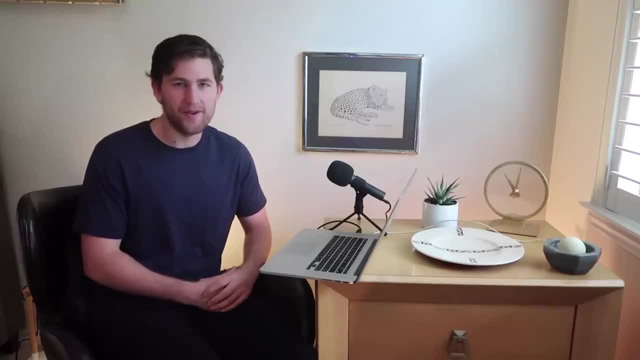 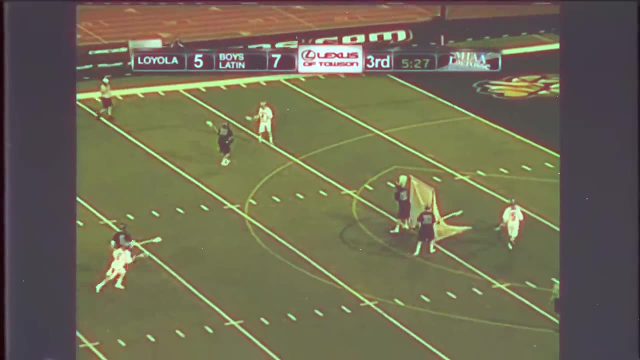 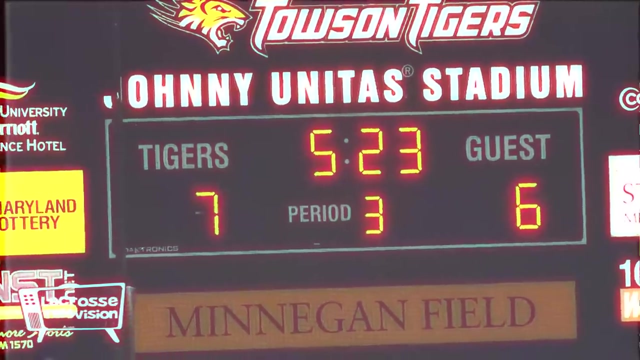 It's anyone's game And someone needs to step up and make a play for their team. So Loyola, trying to cut it to one And look at that. That's exactly what they do. Great assist coming in from Devin McNamara. 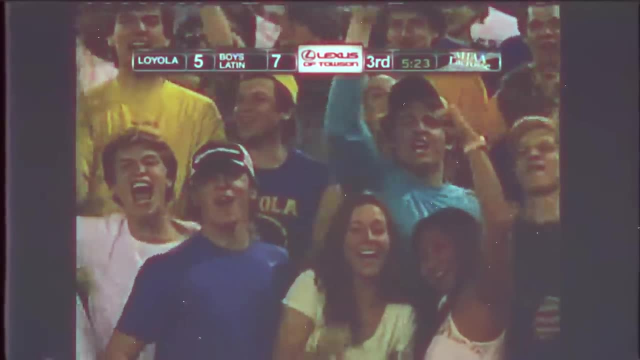 He feeds Alex Rochner in front of the net And suddenly It's a 7-6 game. Well, they've just got two great shots on goal there And they're trying to tie this game. And there's another one. 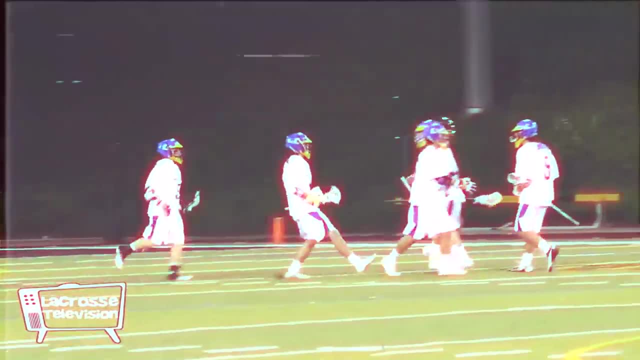 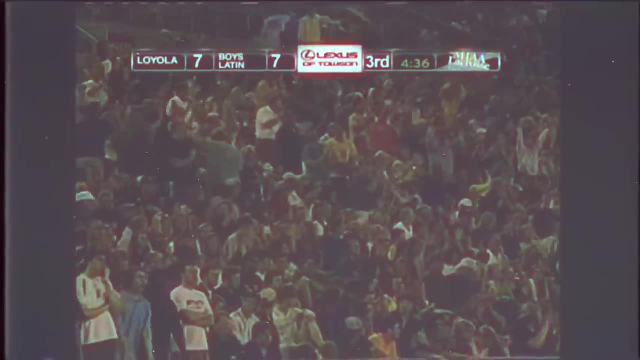 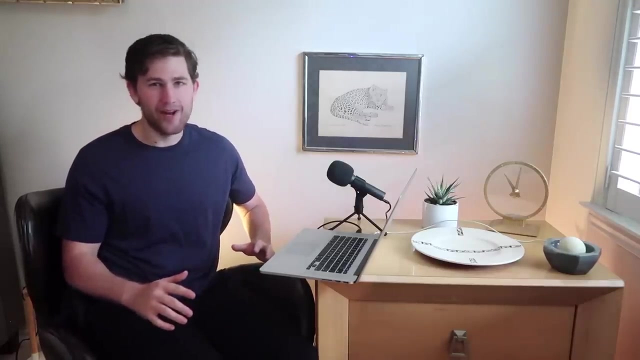 And it's tied. How about that? For Loyola, That was Tim Nordbrook, his third goal of the night. And guess what? We got a tie ball game. And just like that, Loyola has tied the game. That six-goal deficit seems like a long distant memory. 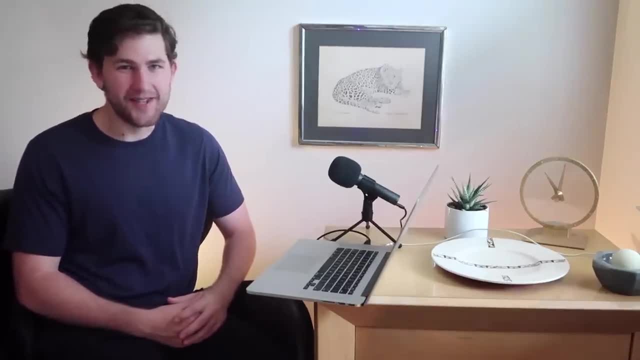 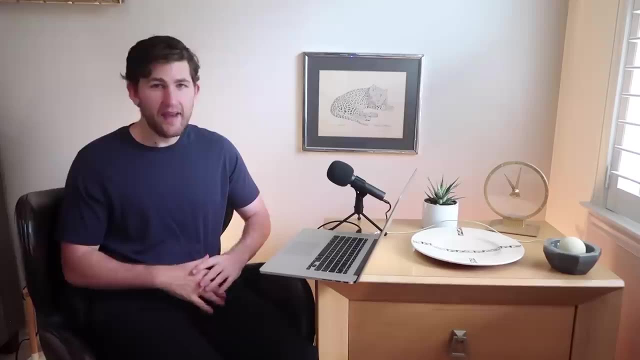 Midfielder Tim Nordbrook is having himself a game And the Dons are feeling it. But hey, there's one more quarter left to play And boys Latin can forget about what's happened so far. If they can just win this fourth quarter, they will be champions. 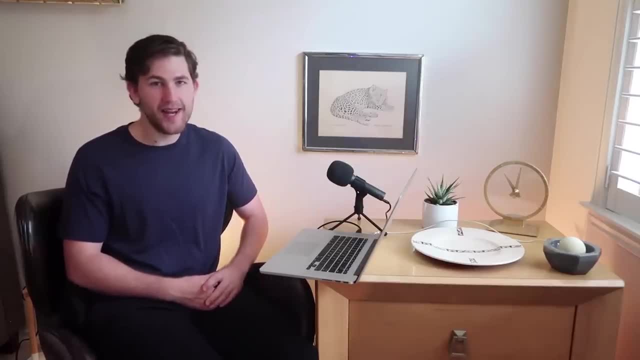 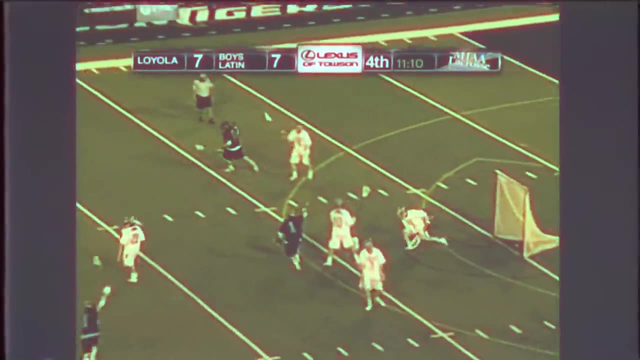 With loads of D1 commits with fresh legs on their sideline, the Lakers can make a run Here and take the lead. This is what you want: a man-up opportunity with the offense you have, And there's the shot And it's good. 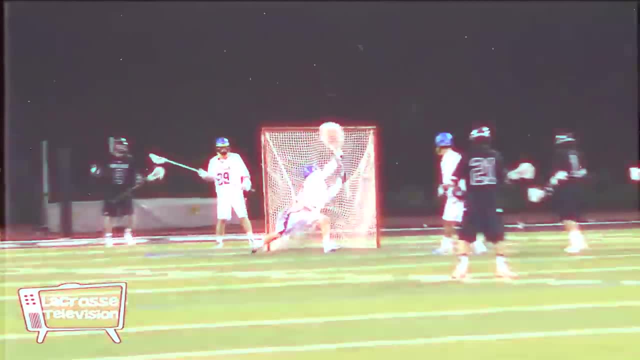 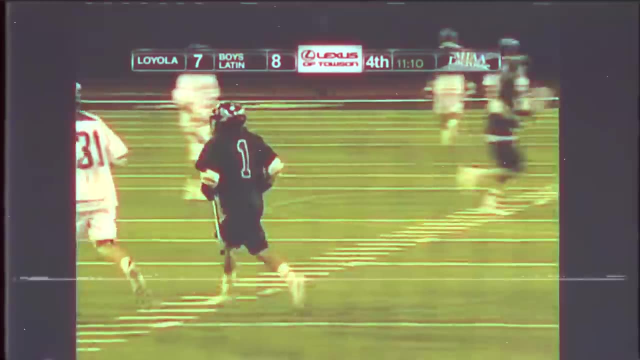 That was Devin Shule, Shule, And that beats AC Newman And boys Latin jumps back out on top Big goal. And again, that just speaks to the depth that boys Latin has Boys Latin here in an open set. 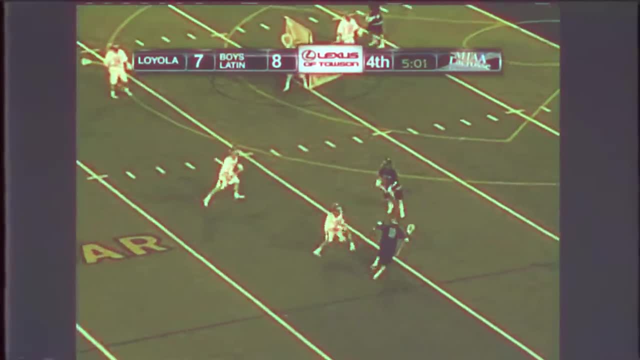 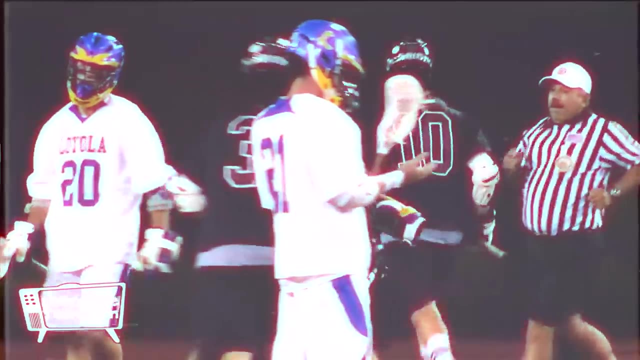 They'll probably jump into something else. And again they're trying to take time off the clock. use possession. They obviously have a good shot or a good matchup. They're going to go Stanwyck, Stanwyck feeds. That would be Michael Lynch. 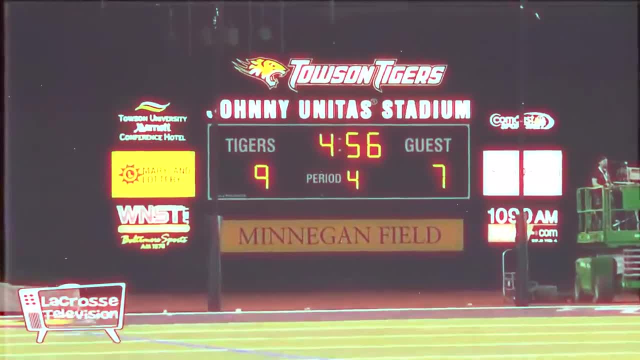 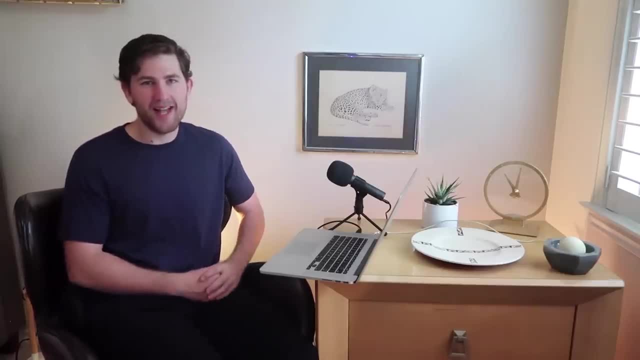 And boys Latin makes it a two-goal lead with 4.56.. And that's Lynch's second goal. It's 9-7 with just under five minutes to play, And boys Latin finally has that momentum back. They can smell a 20-0 season. 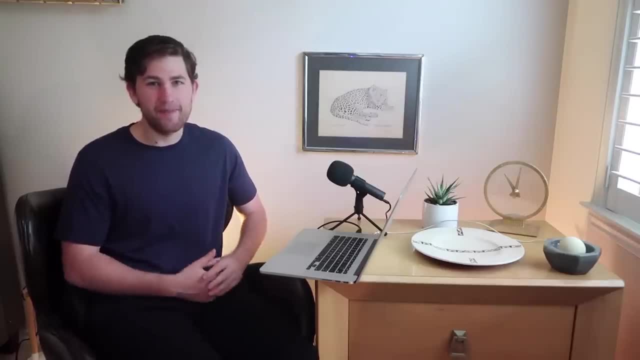 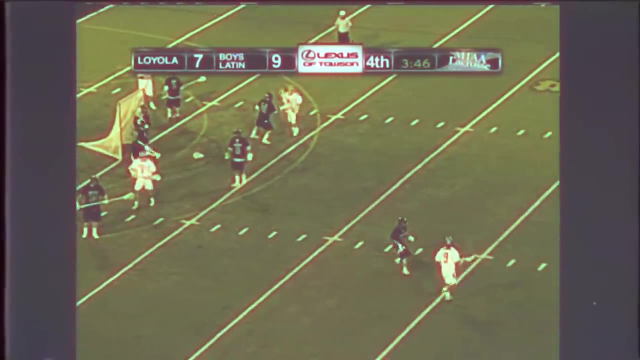 And if they can hold on to the ball for just a few more minutes, this game is theirs. Operating behind the cage, Nowhere to go there. Boys, Latin packs that defense in when they have to. That's Tim Nordbrook, Is it in? 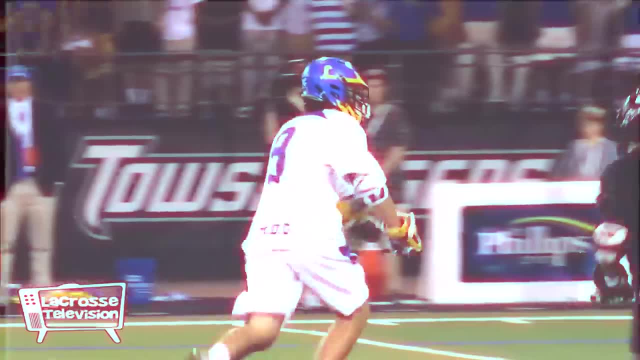 A goal for Loyola, That's four On the night for Tim Nordbrook Boy. you talk about top shelf. huh, That's a great individual effort by him right there to be able to, you know, get his hands free shoot. 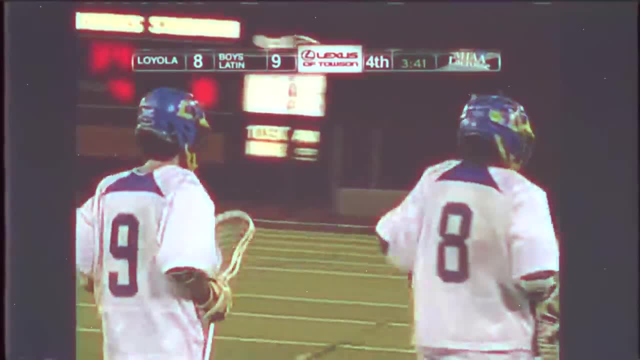 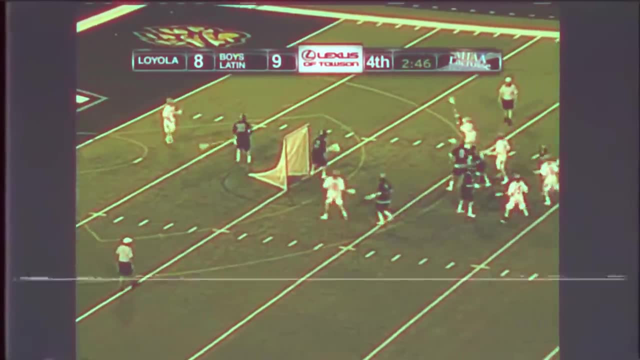 Exactly That's where he puts it in the top of the cage. You know a big goal again to cut it to one here: 9-8, with about 3.40 to go in the game, Ryan Conrad cutting towards the net. 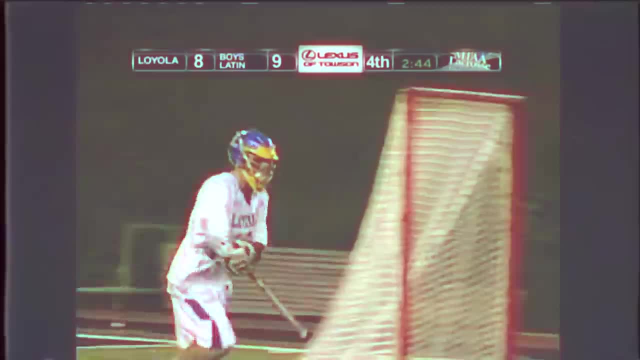 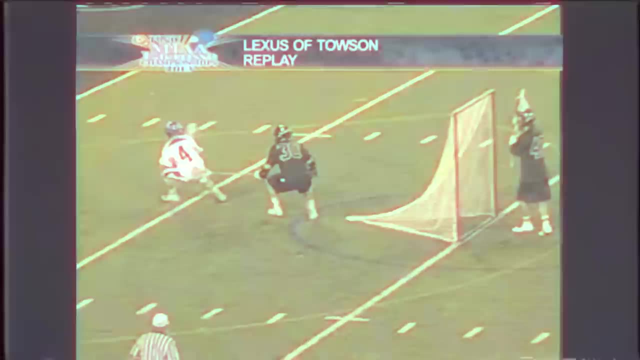 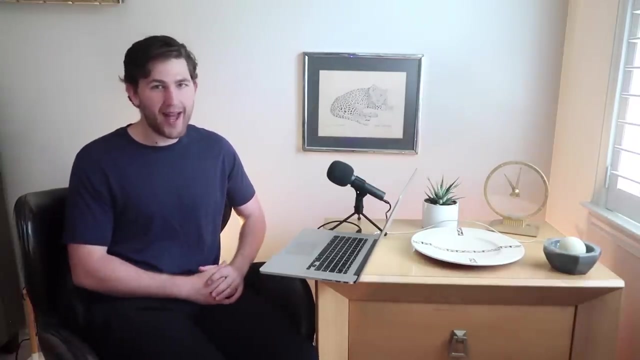 Excellent feed there from Devin McNamara And it's a 10-9 game, Or 9-9 game- Wow, Great. Throughout this year, Loyola's had a mantra that's brought this team together: We fight. Right now they're fighting back and they've tied the game again. 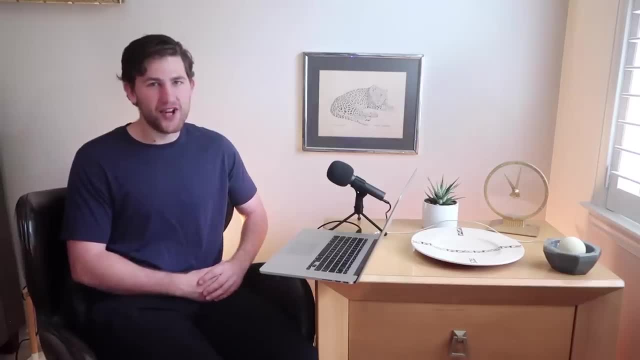 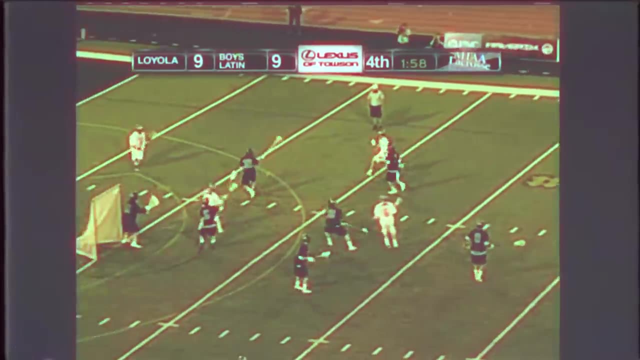 With just under three minutes left to play, one team is going to have the chance to win this game. They would love to go into the old Dean Smith four corners, but they don't let you do that. Look at that inside Fed, right in front of the cage. 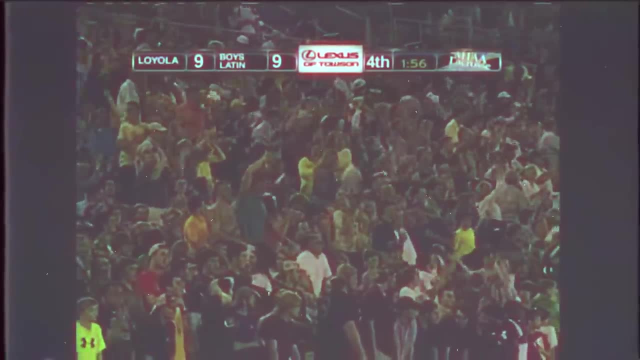 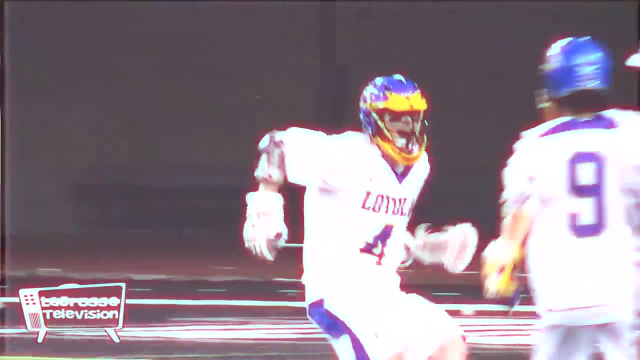 The ball comes into Devin McNamara and he scores And Loyola has the lead. Wow, That's a great play by Tim. I'm not sure. I think maybe because Devin didn't have the ball on his stick, Matt Collins missed him a little bit. 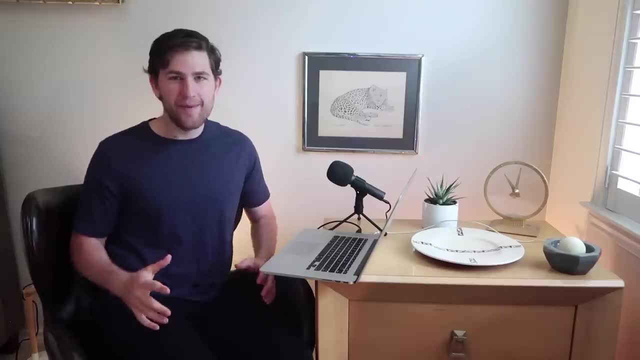 Wasn't necessarily playing, since he didn't have the ball on his stick, And Devin McNamara gives Loyola the lead. The senior is leaving it all out on the field. Wow, This is a remarkable comeback. Wow, The Dons can't celebrate quite yet. 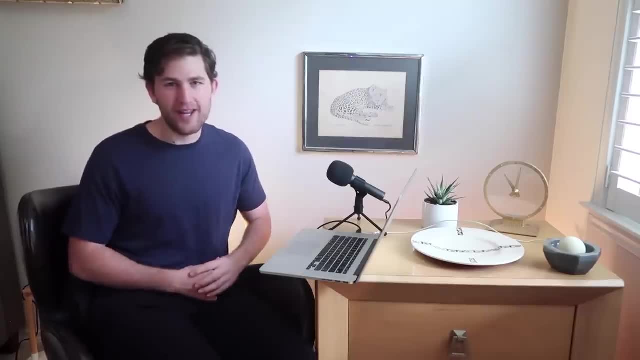 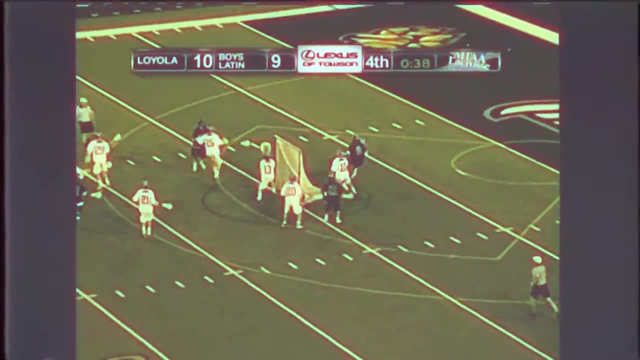 There's still two minutes left to play And Boyes Latin is definitely going to get a chance to tie up this game. It's time for Loyola's defense to make some stops, But I don't know anything like that in a 12-minute quarter game. 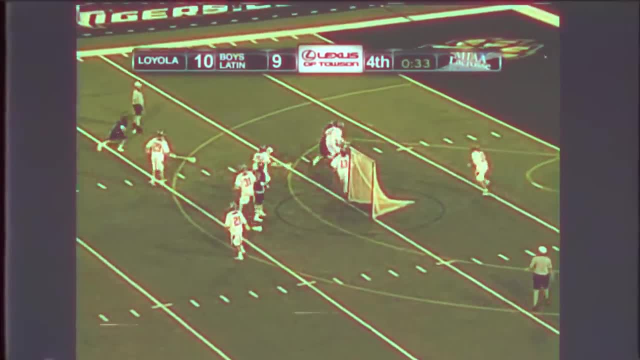 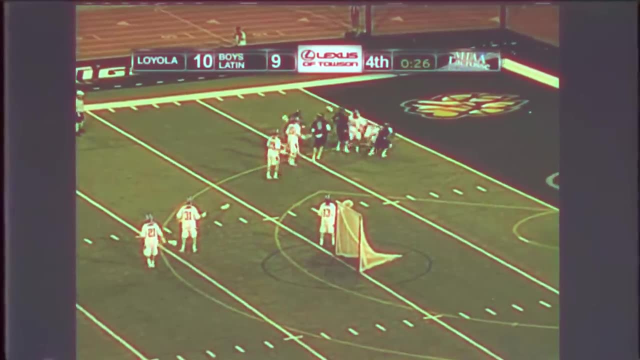 It's six, nothing you know. in the end of the first quarter, Unbelievable comeback. Oh, the stick. The ball came out of the stick for Boyes Latin It's being battled for. The clock continues to run 25 seconds. 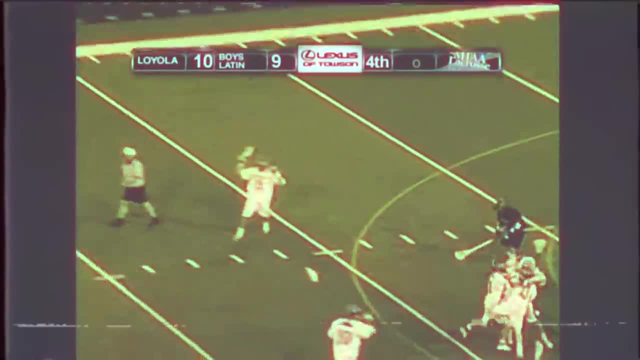 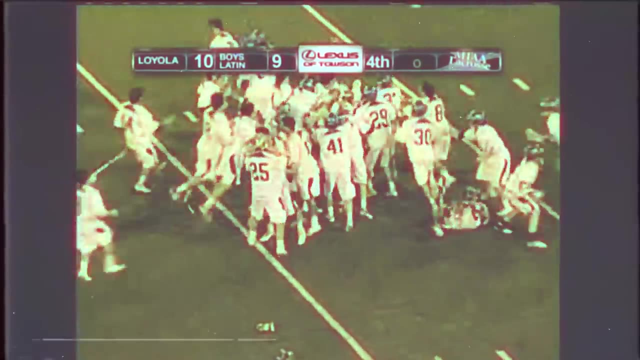 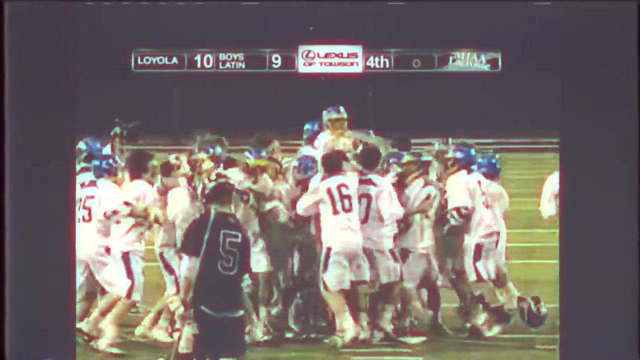 And Loyola's got the ball. Loyola wins The MIAAA Conference in a tremendous upset over the unbeaten number one in the nation, ranked Boyes, Latin Lakers. Ten to nine- your final from Unitas Stadium. Let's just watch this celebration. 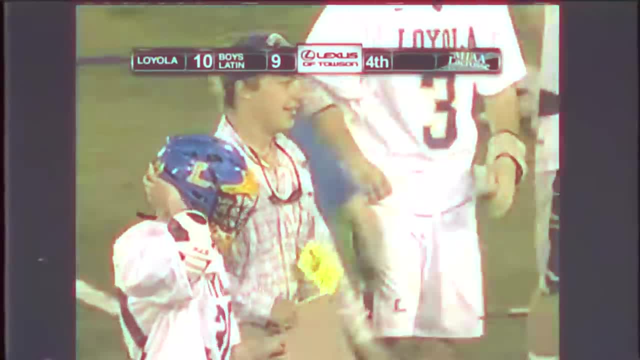 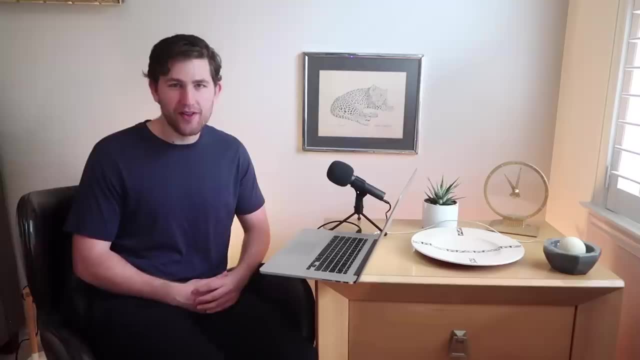 Boy. the faces say it all, don't they? Just a few weeks earlier, most of the team thought their season was over, And now they're at the top of the lacrosse world. This game will certainly go down in high school lacrosse history as one of the all-time greats.